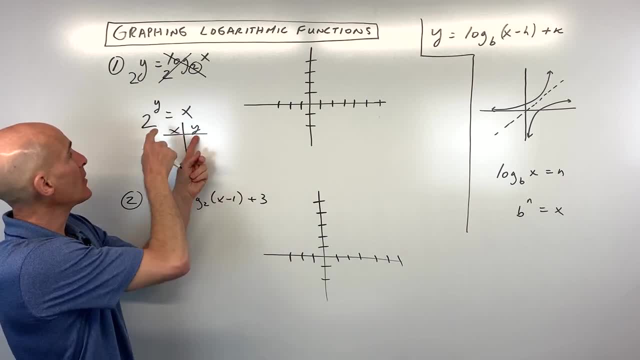 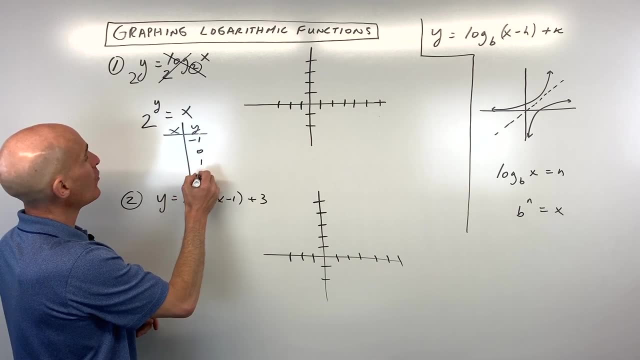 of substituting it for the x values, we're going to substitute in for the y values. It's a little bit easier because y is in the exponent or power position. So let's just go ahead and put in a few values: negative one, zero, one, two. Two to the negative one is one half, because remember when 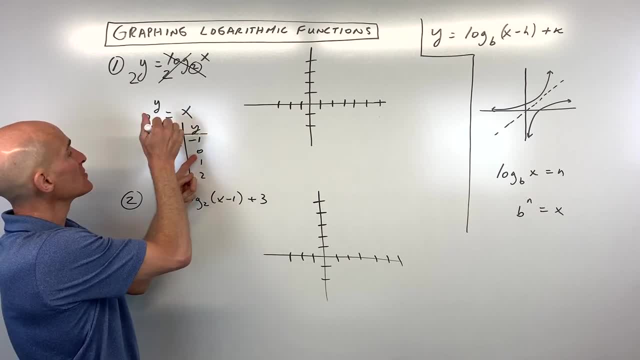 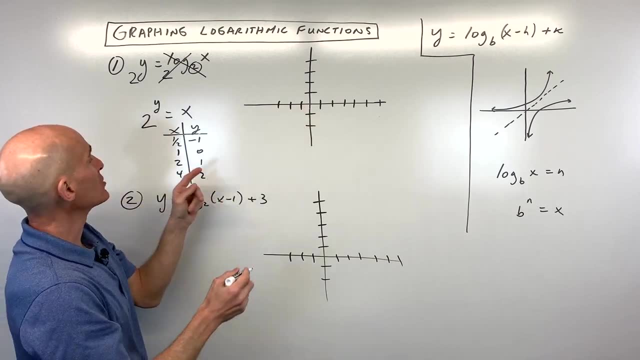 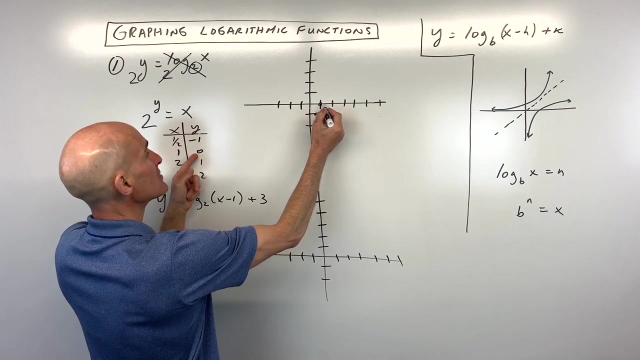 you have a negative exponent. you take the reciprocal: Two to the zero is one, two to the first is two and two to the second is four. Now we're going to plot those points from the origin. So we're going to go right, a half down, one, one comma zero. so we're going right, one up, zero. 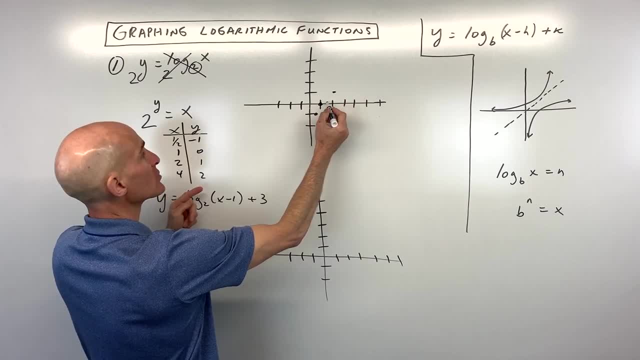 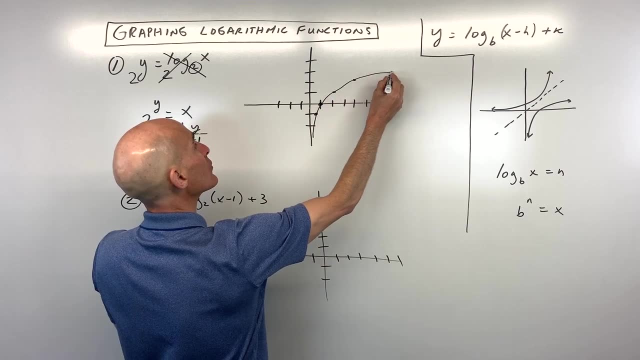 two ones, we're going right: two up one, and then four, two, one, two, three, four up two, And so what you can see here is that the graph is getting you know, it's going up, but it's going up like at a slower and slower rate And it's gradually getting closer and closer to the y. 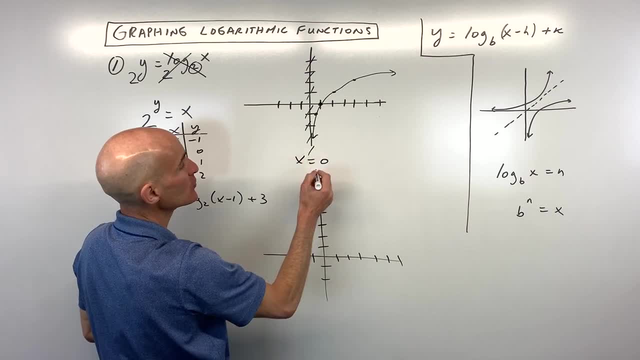 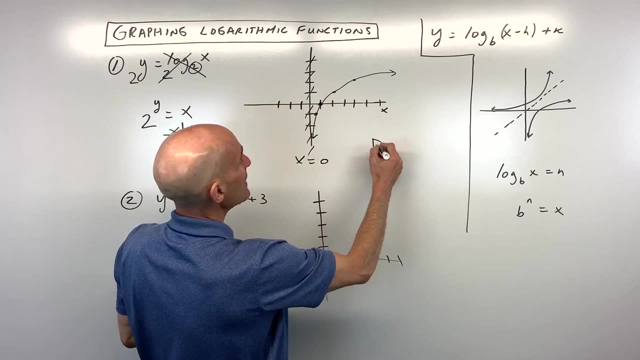 axis. This is our vertical asymptote. It's the line x equals zero. Vertical lines are: x equals lines. So the domain here, what can x be? Well, the domain is going to be: x has to be greater than meaning to the right of, but not equal to zero. So it gets close to zero. 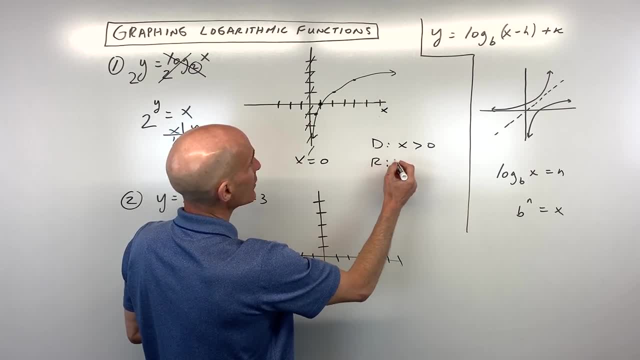 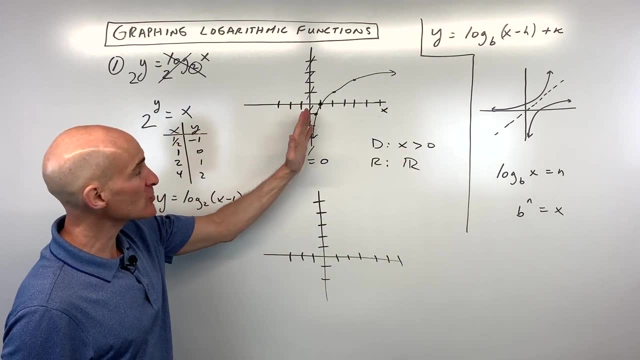 but doesn't touch The range. the y values are going to be all real numbers, because this goes down towards negative infinity. this gradually goes up towards positive infinity. So that's your basic graph. Just remember vertical asymptotes for the logarithms For number two. now we're building on. 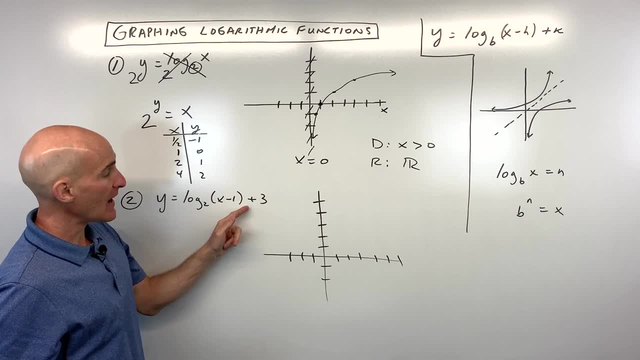 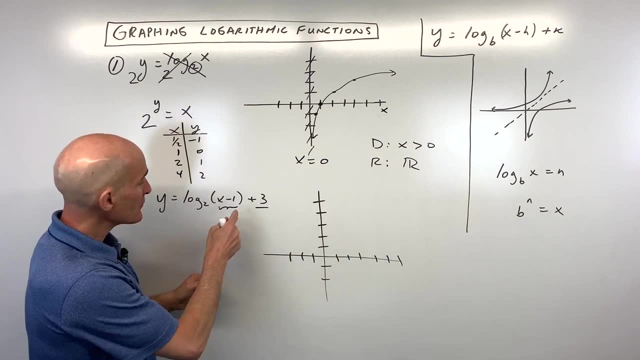 the only difference is see how it's log. base two, but now we have minus one and plus three. So what does this one do to the graph? What does this three do to the graph? What you want to remember is: whatever is grouped with the x here, that's going to shift the graph in the x direction. 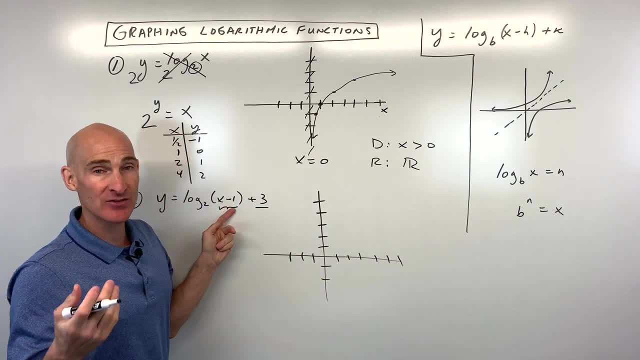 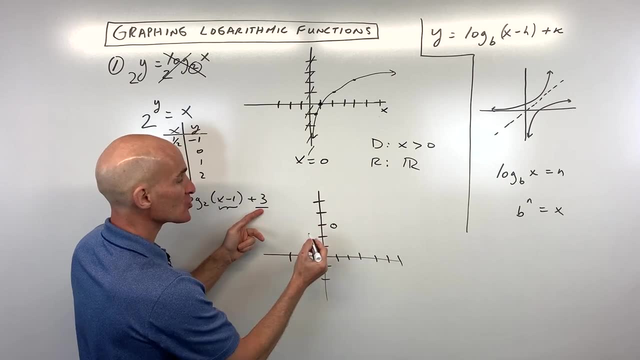 Okay, left and right, but it has the opposite effect. So the minus one is actually going to shift it right one. This one has the same effect. it's going to go up three and what I like to do is just draw like an open circle there. We're going to think of that as our new origin. So this is: 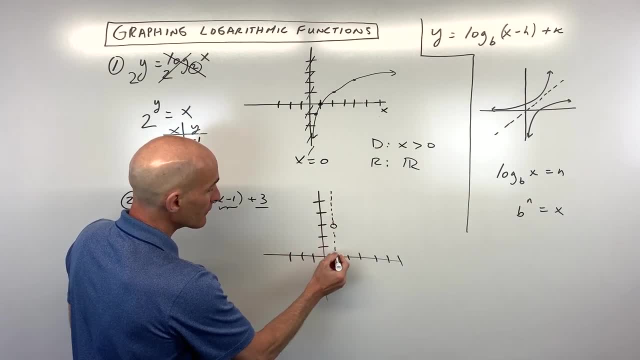 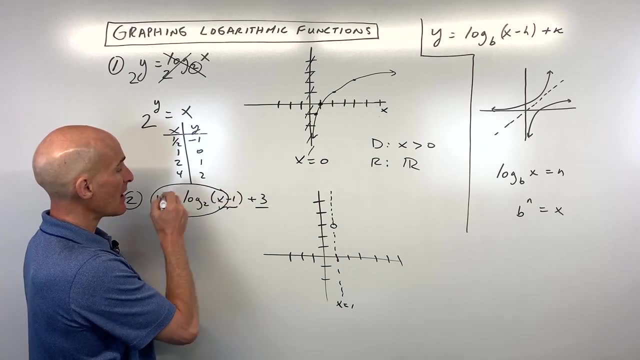 the graph or translates the graph, Then I like to draw in a vertical asymptote. This is the line: x equals one. The graph's going to get closer to that line and then what we can do is we can focus in on this parent function, since we've already taken the shift into account. Y equals log base. 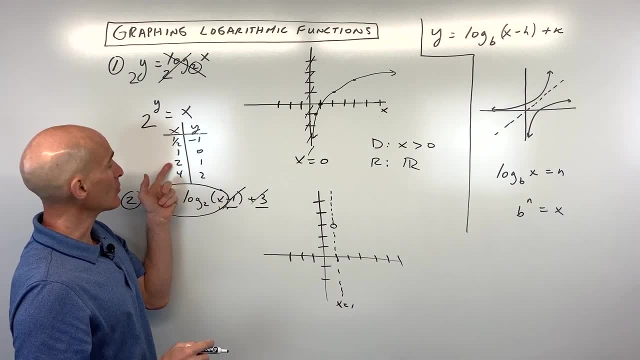 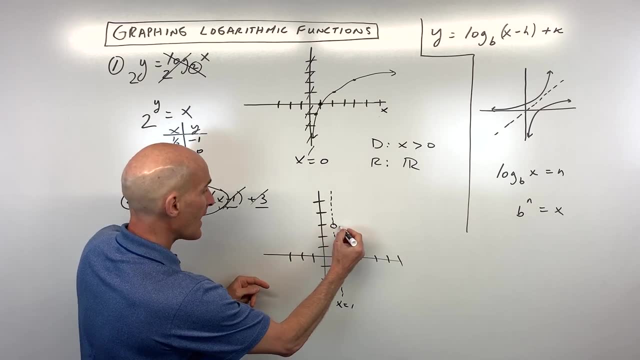 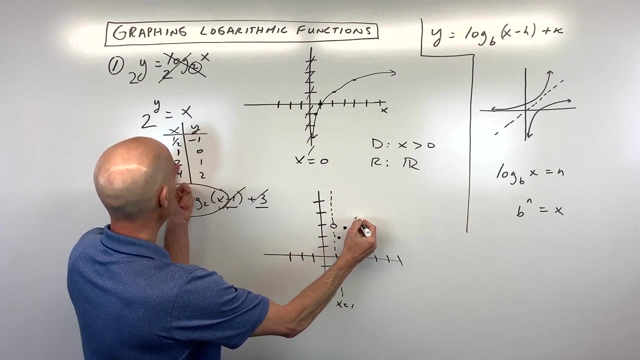 two of x, and that's what we had graphed already or found the points here in this table. So we're going to graph these points from this new starting point. So we're going to go right a half down one, right one, comma zero, a right two, up one, and then right four from this point here: one, two, three, four up two. 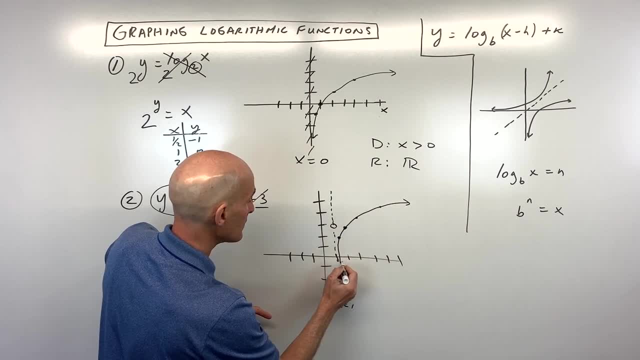 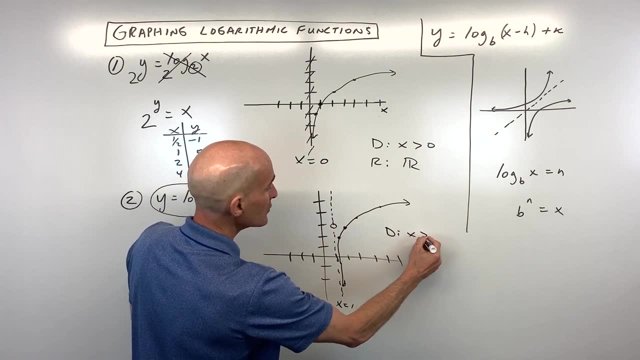 And so you can see the graph's looking something like that and you can see it's getting closer and closer to that asymptote: x equals one. Now, here the domain is going to be: x is greater than one, whereas the range is going to be all real numbers. So you're. 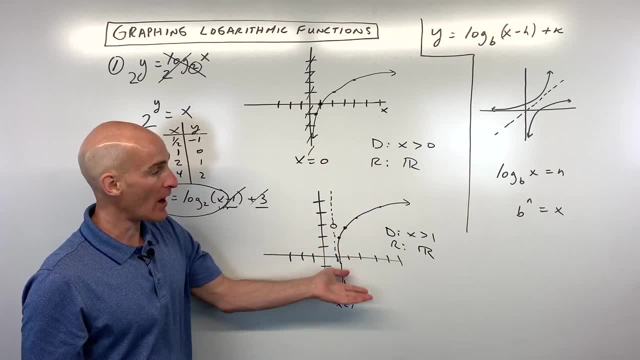 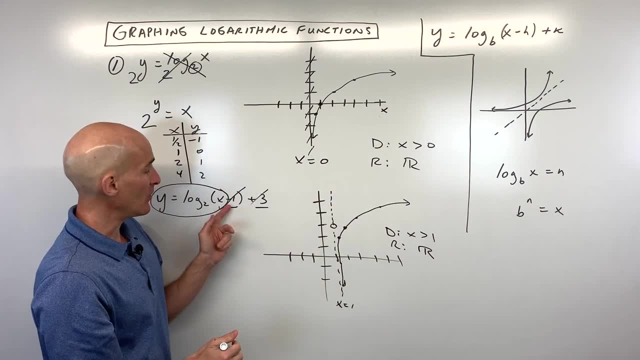 all real numbers, all y values are possible, but the domain is going to be: all real numbers, all y values are possible, but the domain is going to be: you're going to have to pay attention to the shift here and that's this number, here, this group with the x. So let's do two more examples, See if you can. 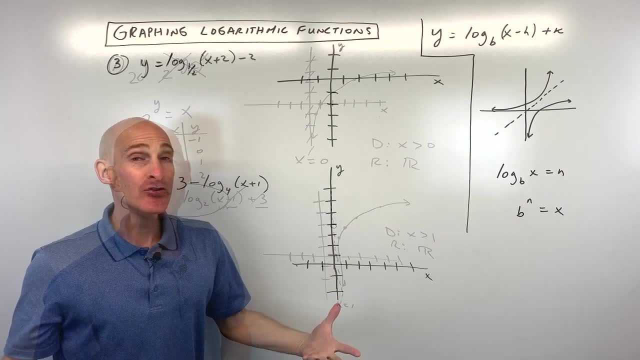 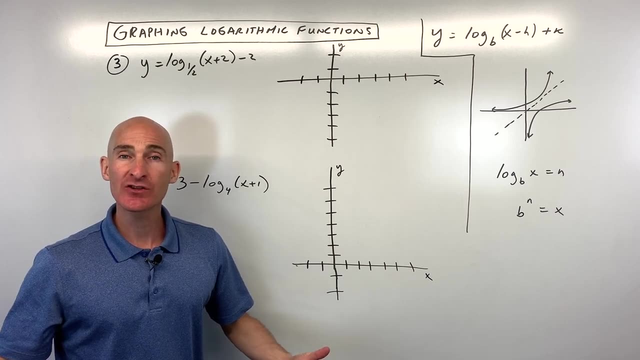 do these on your own and we'll go through them together so you can get some more practice. If you're new to the channel and we're meeting for the first time, my name is Mario of Mario's Math Tutoring, and this channel is all about making learning math less stressful, so you can raise your 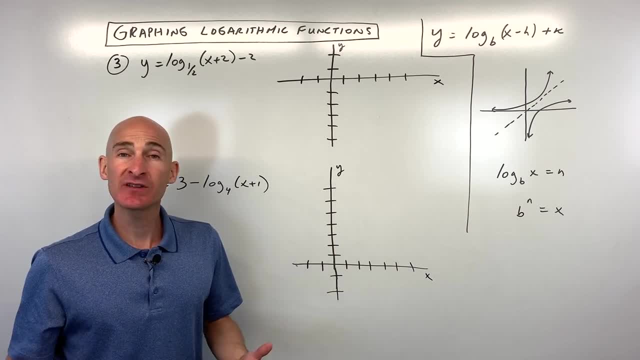 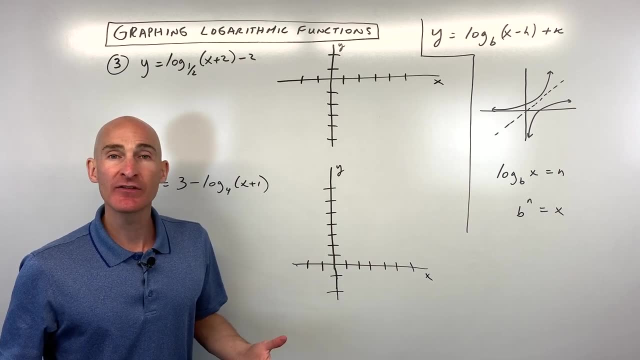 grade, pass your class and go on to pursue your dreams. So if that's something that sounds interesting to you, check out more math videos on my Mario's Math Tutoring YouTube channel, and I've also got math courses available- Algebra 1,, Algebra 2, as well as ACT Math and SAT Math. 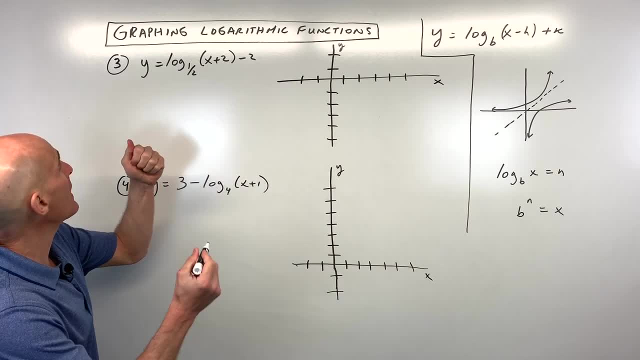 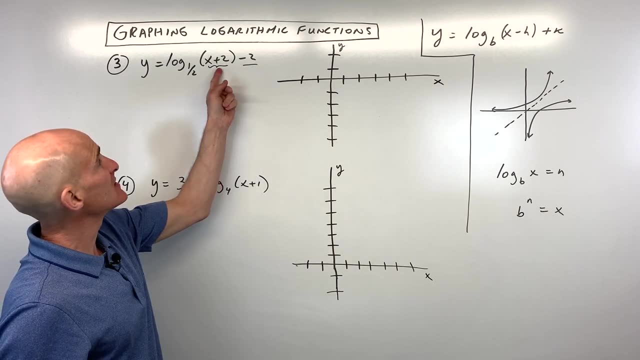 that you can check out if you're interested. So let's go through number three and four together, and the first thing here I like to do is take a look at the translation, or the shift. So in this case you can see this plus two has the opposite effect. it's shifting left two and down two. So 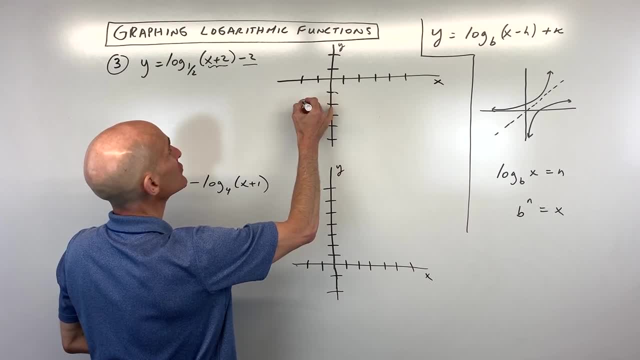 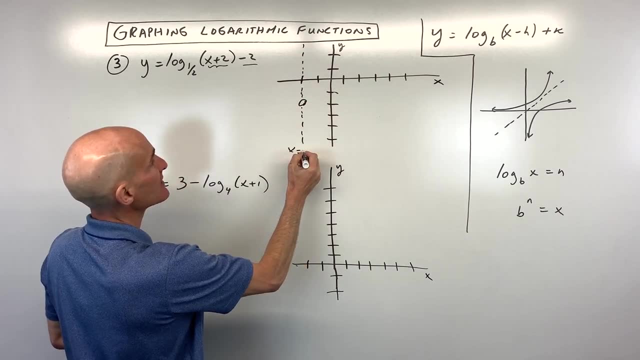 we're going left two, down two. and remember, I like to draw that as like an open circle. we're going to think of that as like our new starting point. I also like to draw in the vertical asymptote, that's the line x equals negative two. and now what we can do is we can focus. 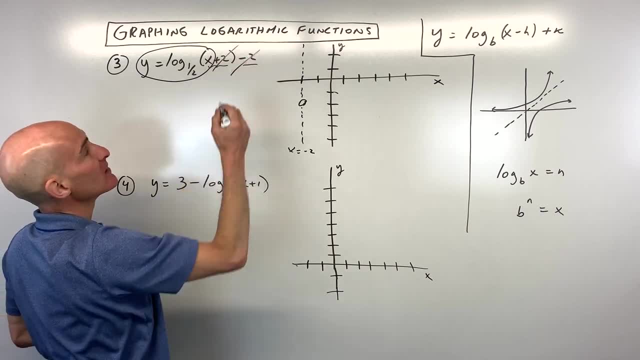 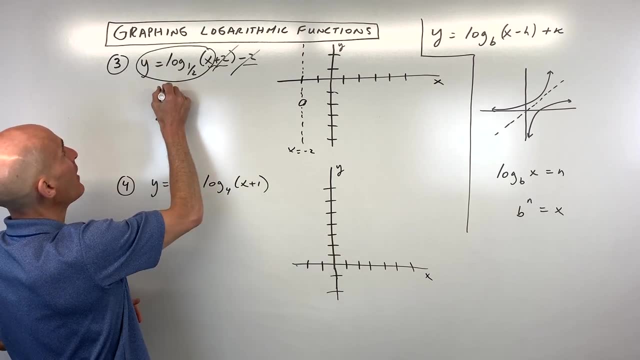 in on the parent function. what's left over after we took that translation into account? I like to rewrite it in the exponential form. remember, this is the base, this is the power, this is our answer. So what we're going to do is we're going to make a table of values, but remember, instead of 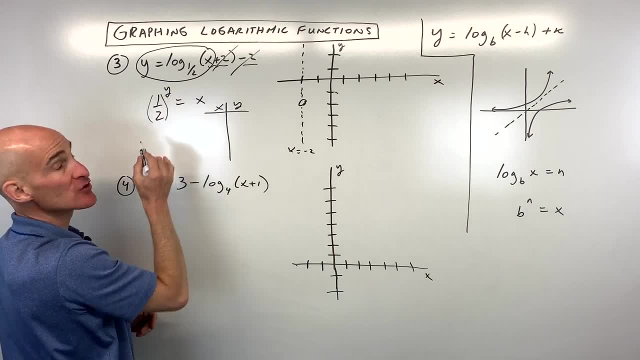 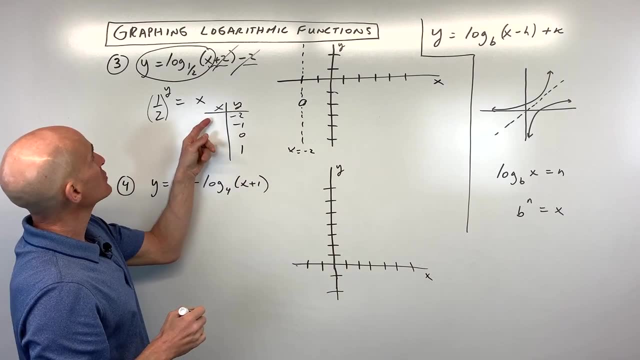 substituting it for x. we're going to substitute it for y. that's a little bit easier because we'll use y as in the exponent position. So let's go ahead and put in negative two, negative one, zero one. So if we put in a negative two, one half to the second, I'm sorry, one half to the negative two. 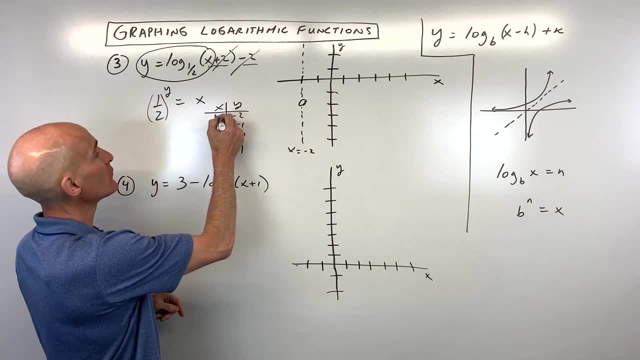 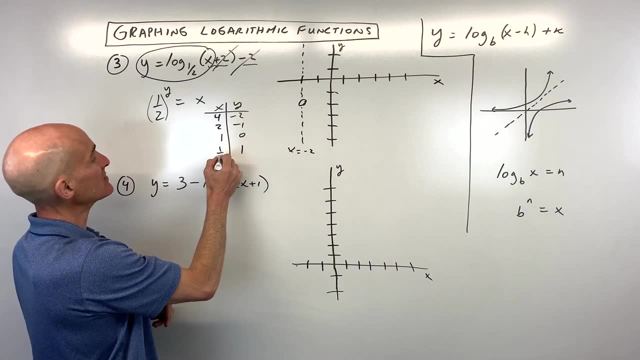 the negative, you take the reciprocal, so that'd be like two. and then two squared is four: one half to the negative one, you take the reciprocal, that's going to be two. anything to zero, power is one. anything to the first, power is itself. So when we graph these points from the new starting point, 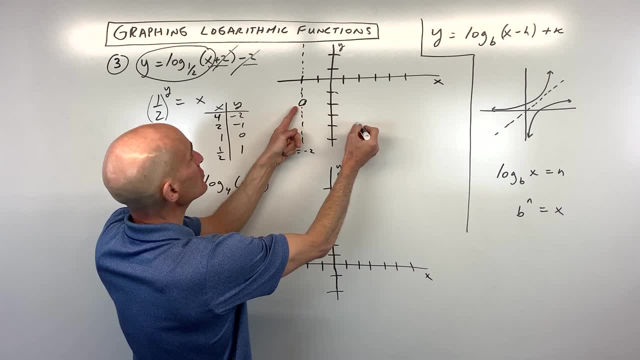 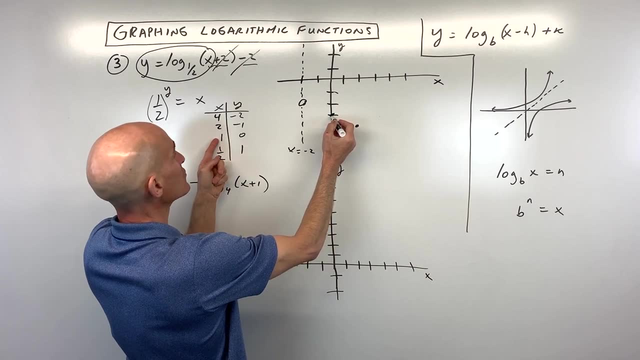 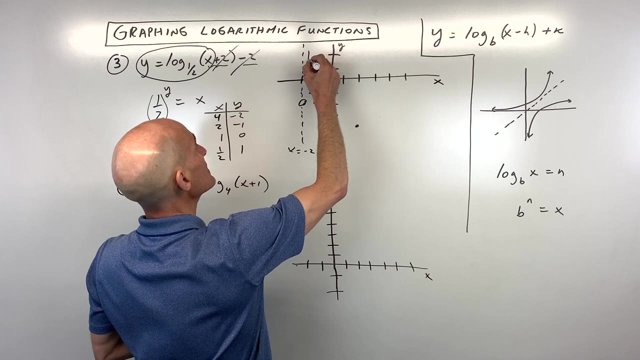 we're going to go right four down two, which is going to be right about there. right two down one, and this one is right one down zero, and then right a half up one. So here what you can see: a little bit different law graph than we're. 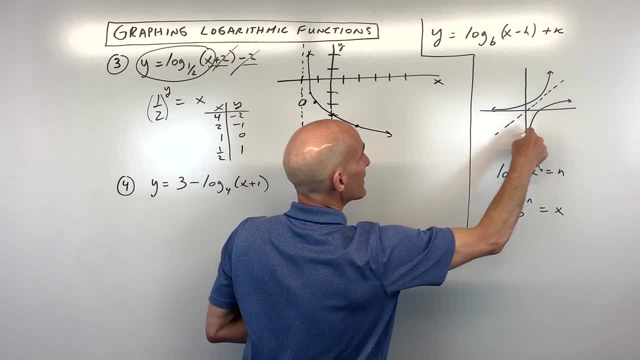 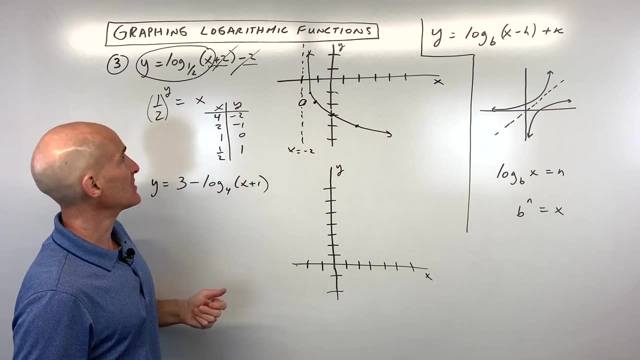 used to seeing it's going like this instead of like this. and why is that? Well, it's because this base here is between zero and one Okay. so if it was like a half or a third or fourth, you're going to get that type of shape, as opposed to the other way around. So you're going to have a little bit. 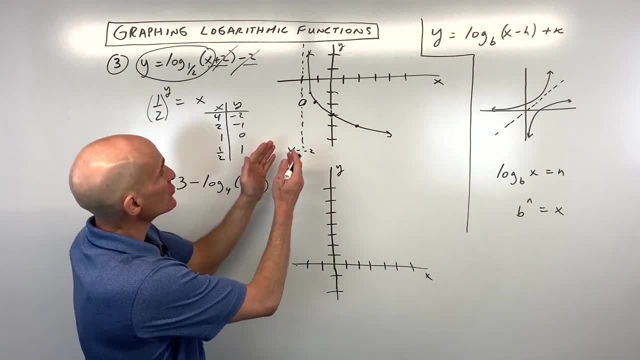 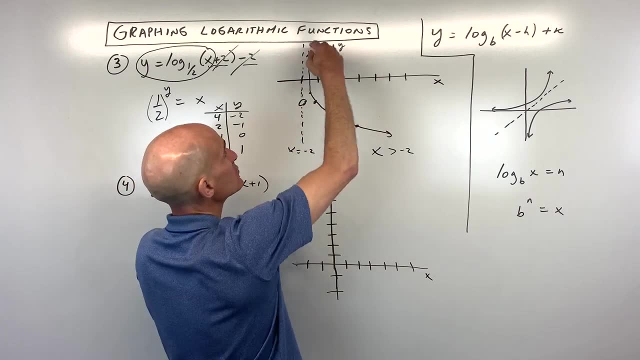 to that type of shape there. So in the case of the domain, the domain is going to be what x can be. x is going to be greater than negative two. our asymptote is: x equals negative two, and then our range, we said, is all real numbers. So number four: see if you can do this one, this one's probably the most. 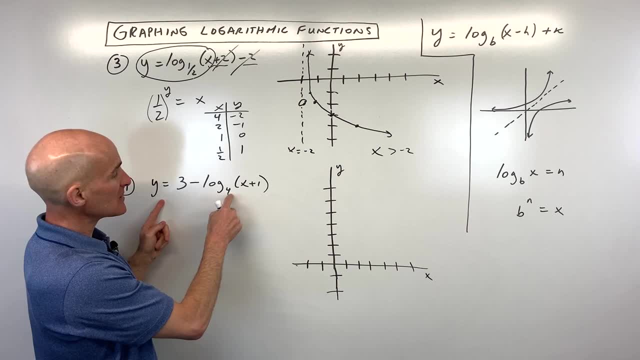 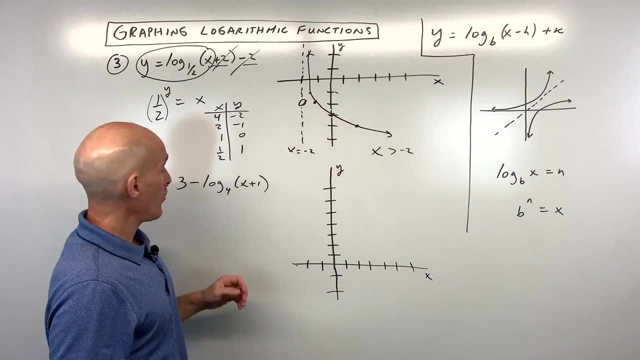 challenging one we've done so far. y equals three minus log base four of the quantity x plus one. Well, you might be saying: well, Mario, this doesn't look like it's in that form. Well, you see, this three here, this three, we can move over here. So this: 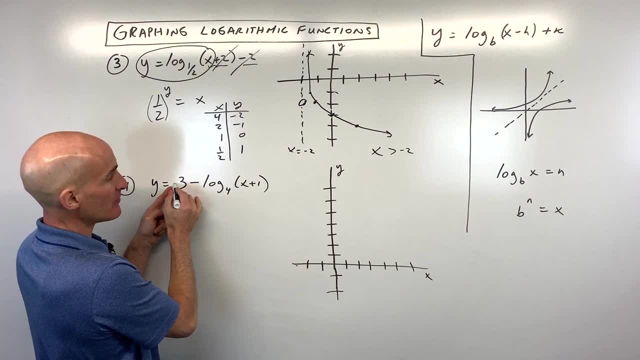 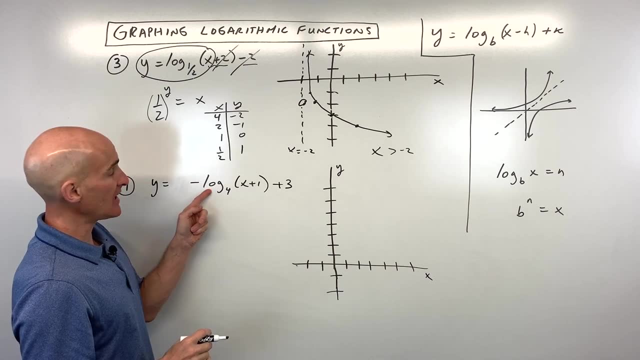 is a positive three. right, see, there's nothing to the left of the three. that means it's a positive three, which is like plus three, and now I'm just going to erase this. Okay, the negative still stays here. this is a negative log. What do you think the negative does to the graph? Well, you're. 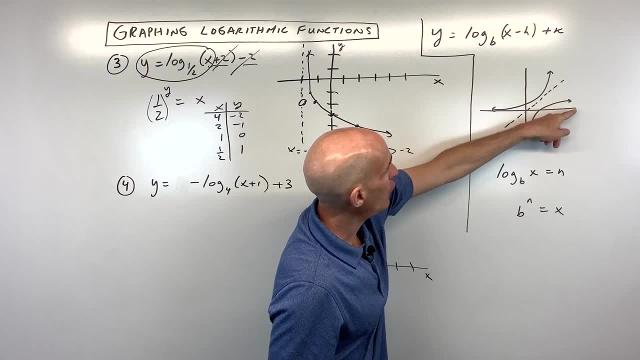 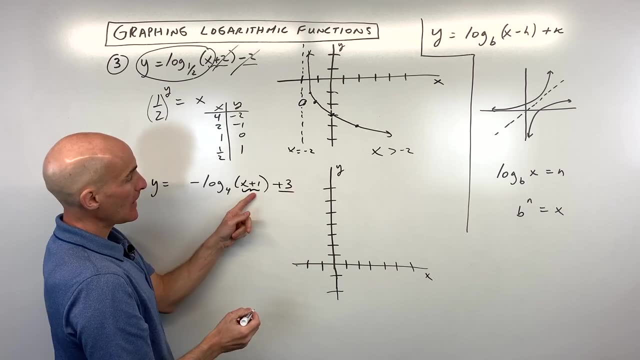 making all the y values the opposite. it's going to reflect it over the x-axis, But let's go ahead and follow the pattern we've been doing so far, which is taking the shift into account first. We're going to be shifting, not positive one, but to the left negative one. this one's the opposite. 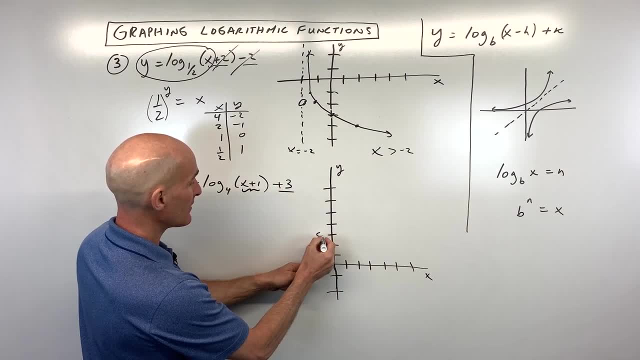 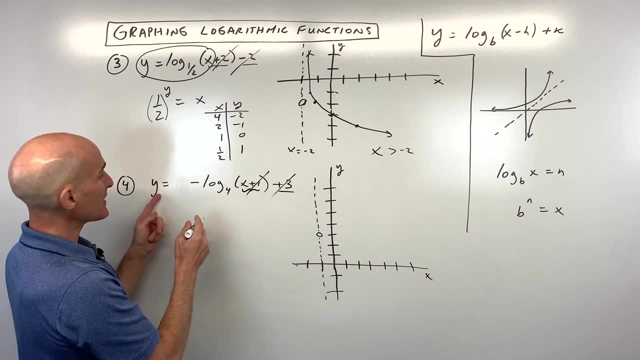 Plus three, it has the same effect. we're going up three. So we're going to think of that as our new origin or our new starting point right Now. we've taken that into account. so now we're down to this parent function. y equals negative log base four of x. See this negative here. let's go ahead. 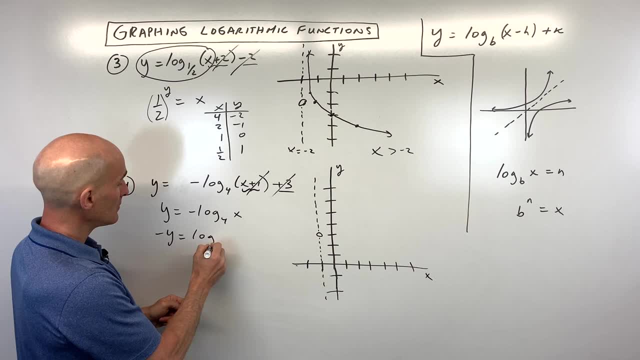 and multiply both sides by negative one, just to get this log by itself. and now we're going to rewrite it in the exponential form. Remember, this is the base, this is the power and this is the answer. So what we're going to do is we're going to multiply both sides by negative one, So we're. 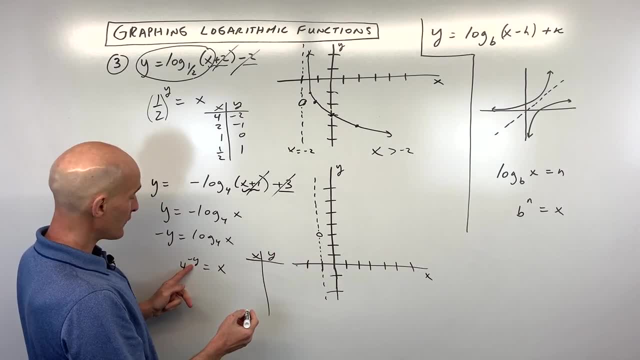 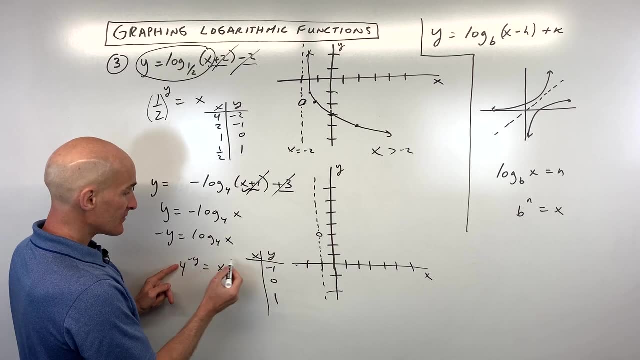 going to do is we're going to make a table substituting values in for y, not x. So negative one, zero one. let's just try those three, So four to the negative times. negative one, that's like four to the positive one, which is four. Four to the zero, which is going to be one. Four to the negative one. 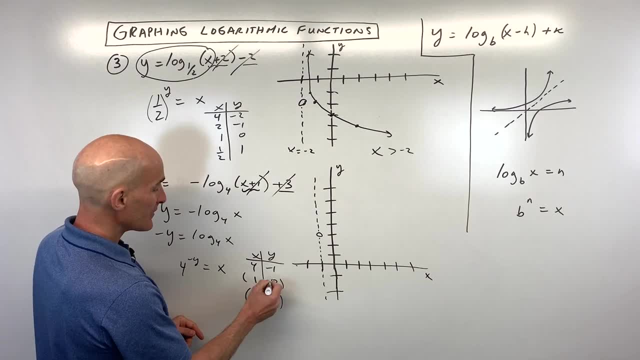 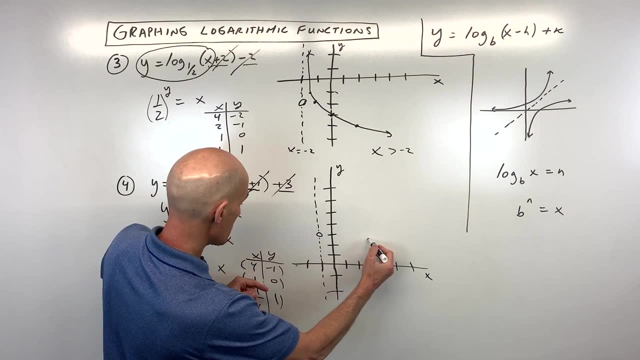 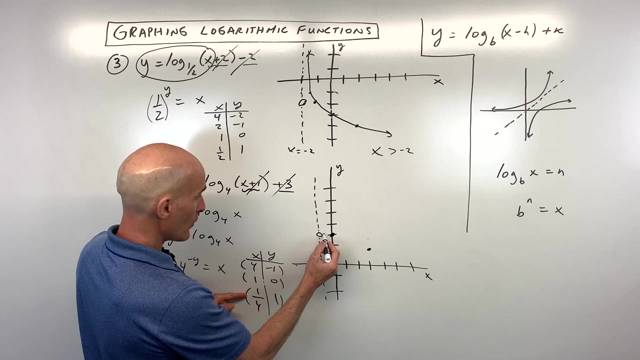 remember the negative. you take the reciprocal one fourth. So we're going to plot these points now from our new starting point, our new origin. So we're going to go right: four. one, two, three, four. this is going to be right about there. One zero, so write one, but up zero and then write one fourth. 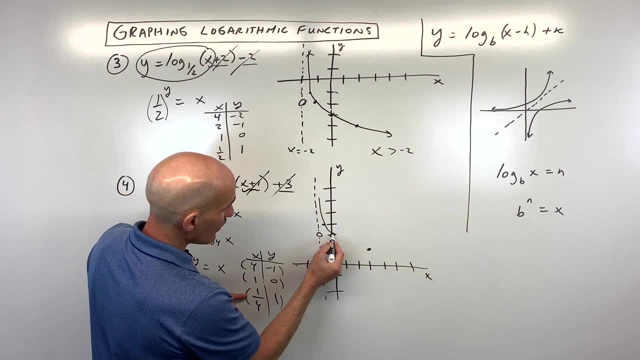 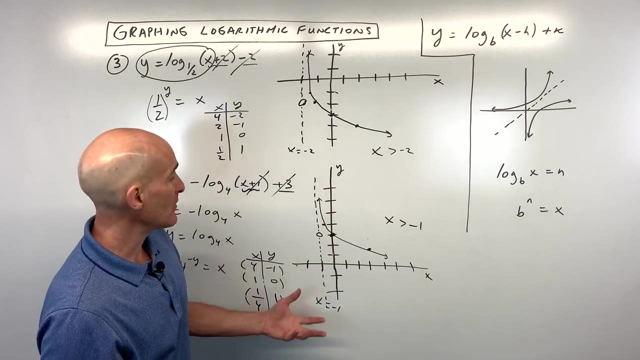 up one and there's our graph like that and it keeps going down, down, down, like that, up, up, up. So the range is all real numbers, but the domain is going to be: x is greater than negative one and our vertical asymptote is x equals negative one. So that was a challenging one If you want to see.